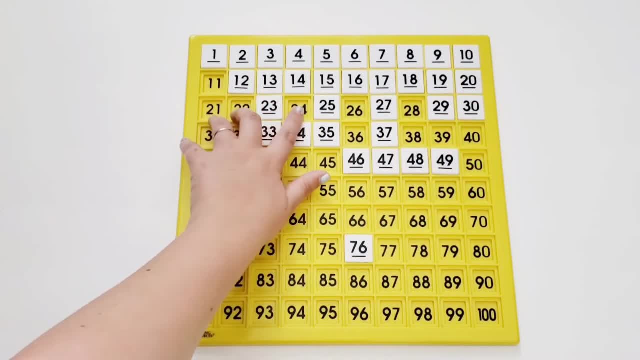 our 20s are going to be here, but the ones place changes by one, goes up by one, Okay, and then they're going to notice that all of the ones place numbers, so all of our fours in the ones place, are in a vertical row, Okay, so again, it depends on you if this 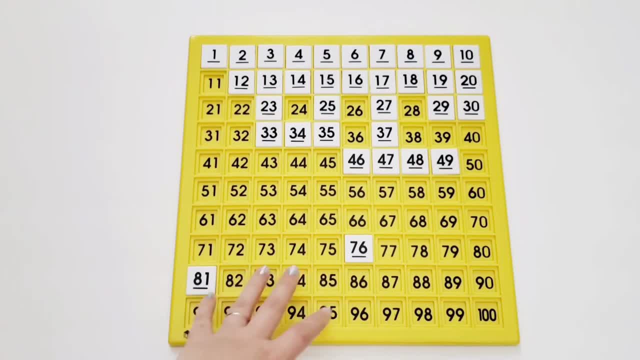 is something you have to teach, or maybe you just kind of discuss it, as you guys are plugging in numbers. So I know that the eights are over here, and I know that the twos are over here, And so that's going to make plugging in the numbers that much faster. Oh, here's. 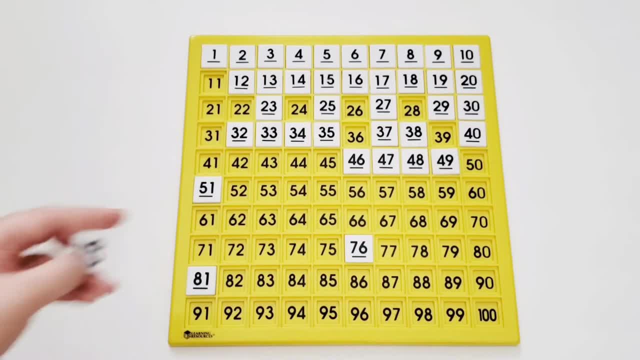 a 10,, a 40,. that goes over here all the way at the end, and I know that, And so this is something that might just have to be worked through naturally, or it might have to be a lesson, but it's definitely something that needs to be learned to make plugging in the 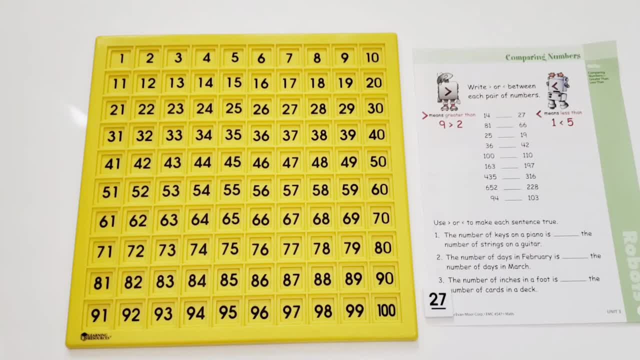 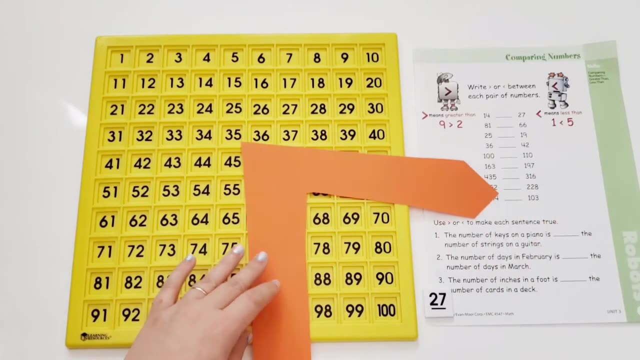 numbers that much quicker. The next concept we're going to work on is greater than and less than. Now you might have to bear with me as I try to explain my method here, But what I have done is just cut out this little arrow here, our symbol for greater than or. 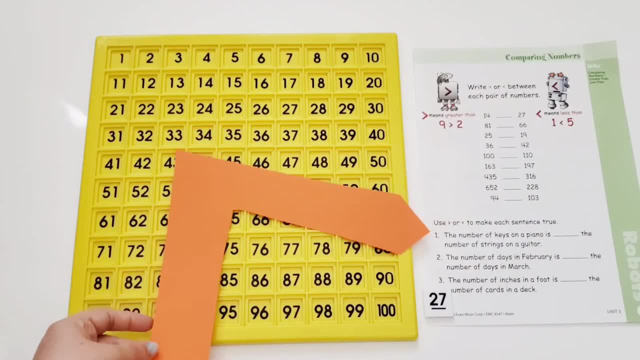 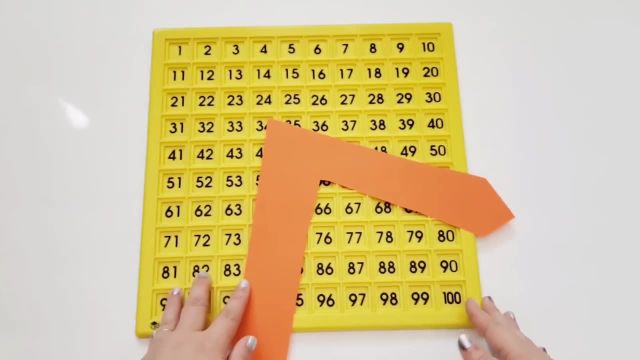 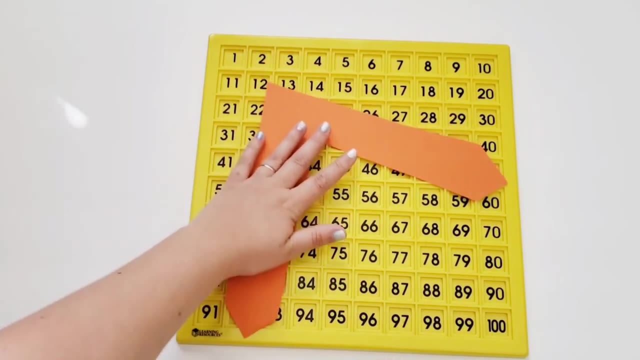 less than to use as a visual for them to understand this concept, And so what I'm going to do, before we even get to any worksheet, is just explain to them that any of the numbers down here are going to be bigger than any of the numbers here. So here's our big side. 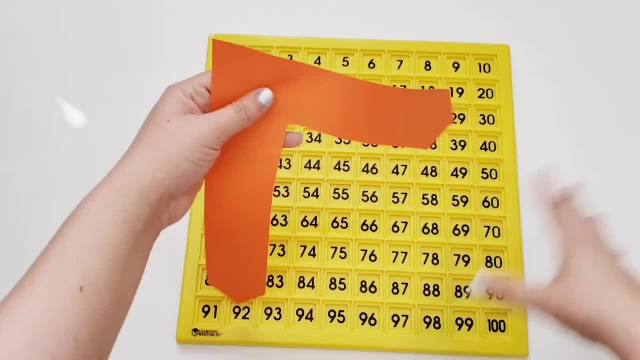 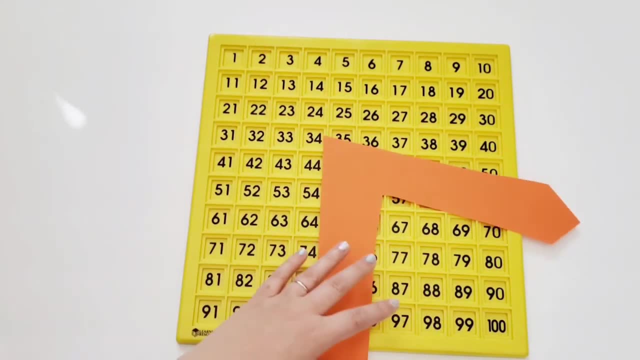 of our arrow. okay, This represents that big numbers are down here and smaller numbers are up here, And so this is just going to be our guide And we're going to have it kind of a diagonal here, just because if we're talking about what numbers are bigger, just. 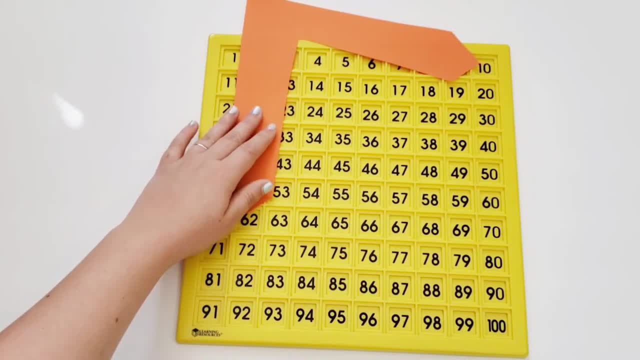 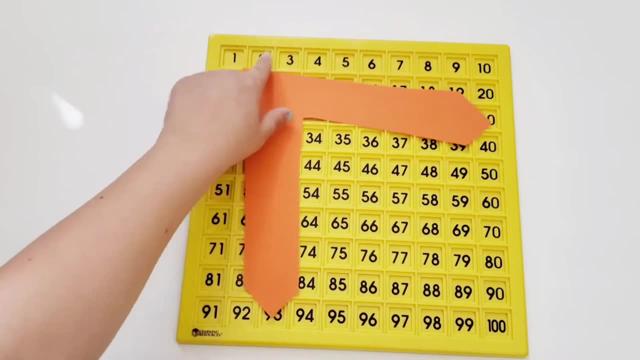 in one row. So if we're talking about seven bigger than three, they need to know that the larger end of the arrow is down here and the smaller end is over here. So, yes, we know that seven is bigger than three. So let's just talk about, even if we didn't have this, even if you didn't- 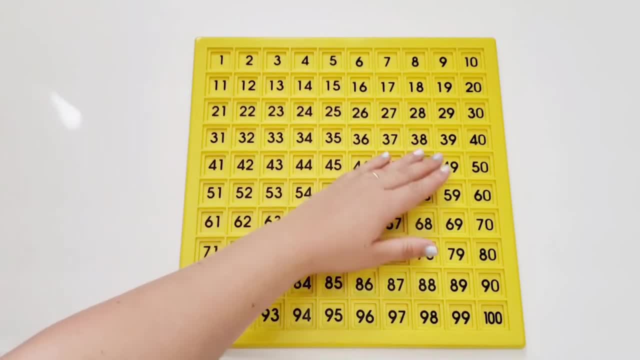 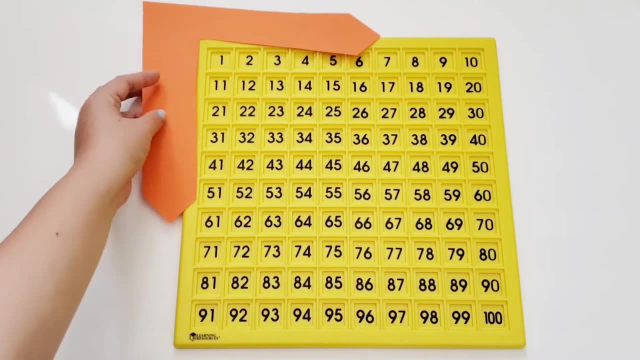 want to cut that out. let's talk about that as you move down the board. these are all bigger than anything up here, okay, And so this is just going to help them remember that, So we might even just keep it up here in the corner for them. Let me pull it down, so you. 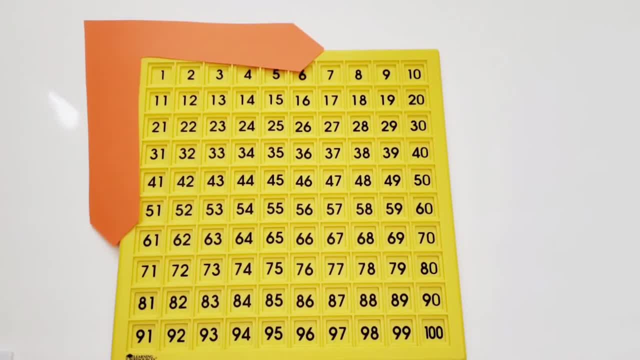 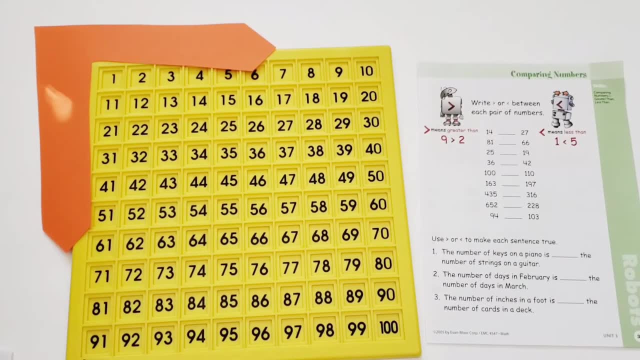 can see it, But just as a reminder for them. And so now I happen to have a worksheet again that I just pulled out of a workbook we have. It's not something you need to do, but if you wanted to work on this concept. our first problem here is 14 and 27.. So let's plug in those. 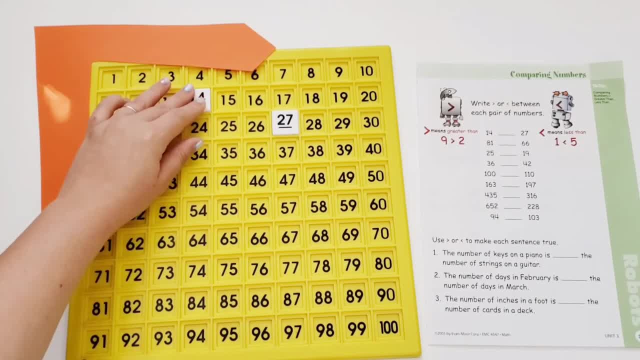 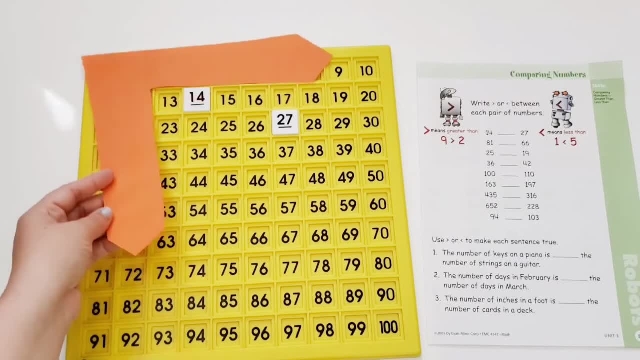 numbers. I happen to have these tiles right here, So we have 14 and 27.. So now let's look at our arrow here Again, I just cut this out of an orange paper that I have nothing fancy construction paper, whatever you have. 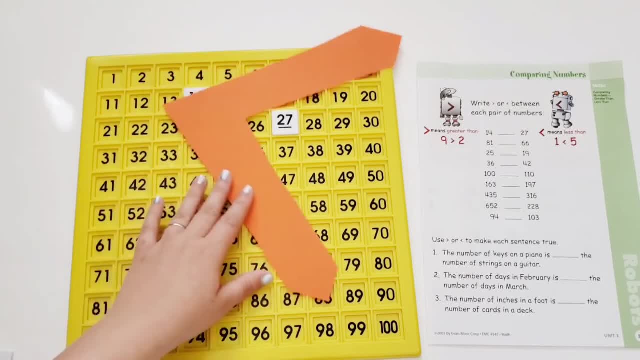 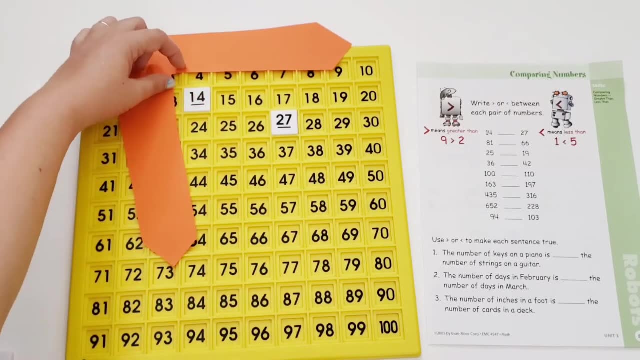 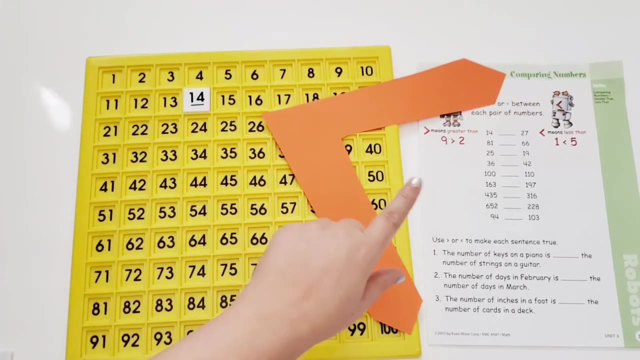 And so they can see with our arrow here that 27 is definitely on the bigger end of the arrow and the 14 is closer to the pointy end. okay, So the bigger number has to be 27.. And so then this will show them that this is the way the arrow goes when you write it in. So 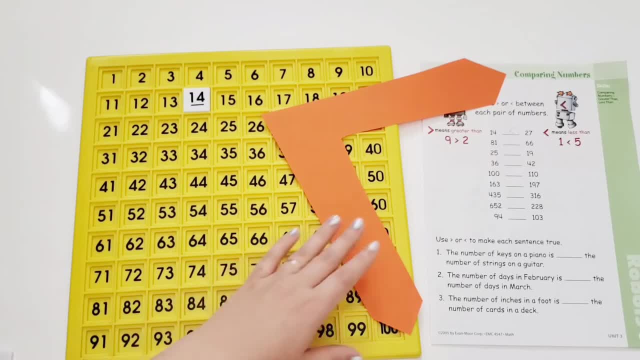 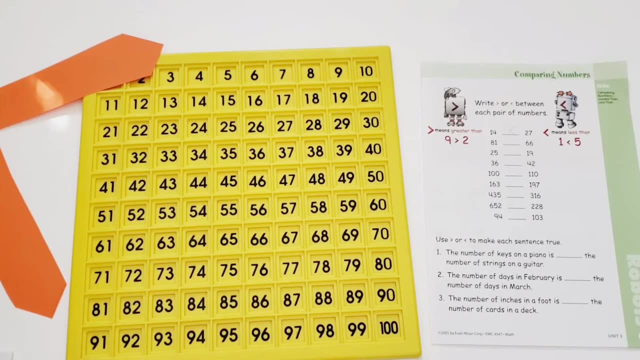 27 is bigger than 14.. Okay, let's move on to the next one. We have 81 and 66.. Now I don't want to look for these particular tiles. I don't want to look for these particular tiles, so this time I'm just going to switch to the translucent ones. so we have 81 and then we 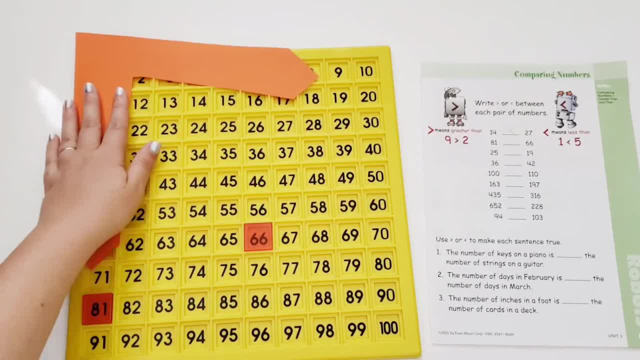 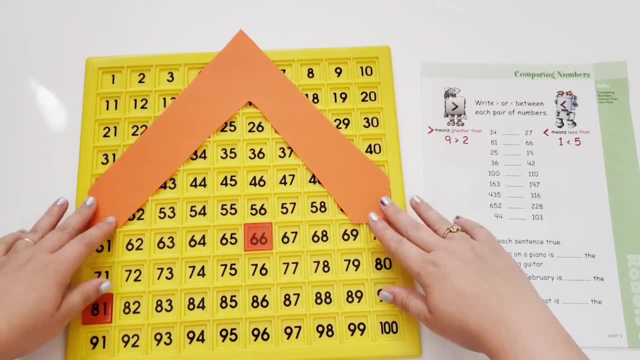 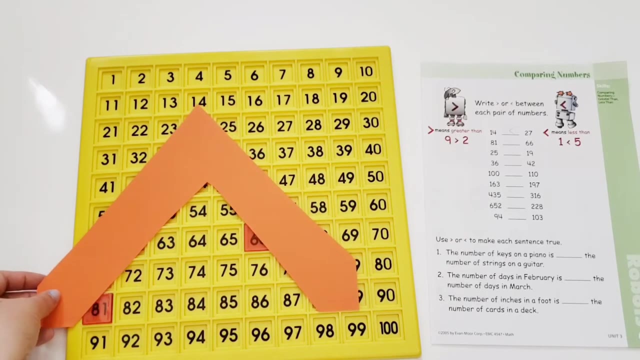 have 66, okay. well, if we have our arrow here now, it's facing a little bit differently, okay. so let's just tilt the arrow to make sense with where the numbers are. okay, the arrow is on the bigger end. let's line it up so that they both fit within the arrow. the 81 is on the bigger end of the arrow. 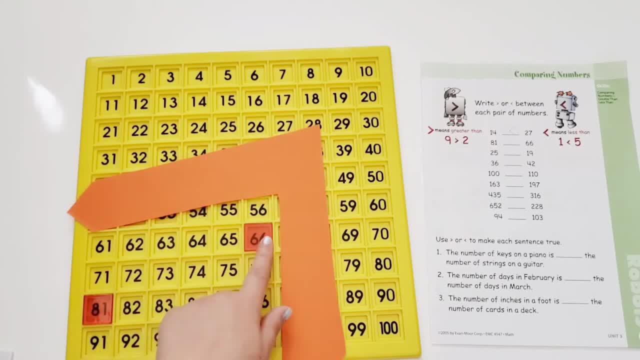 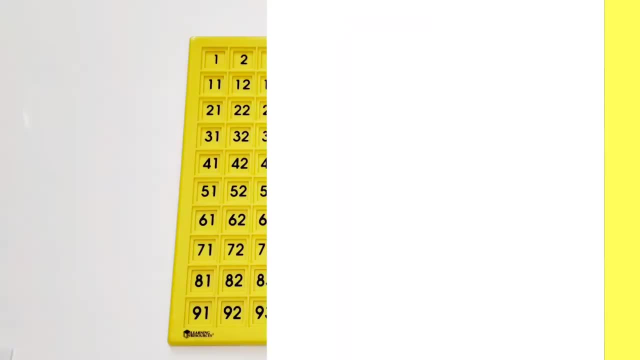 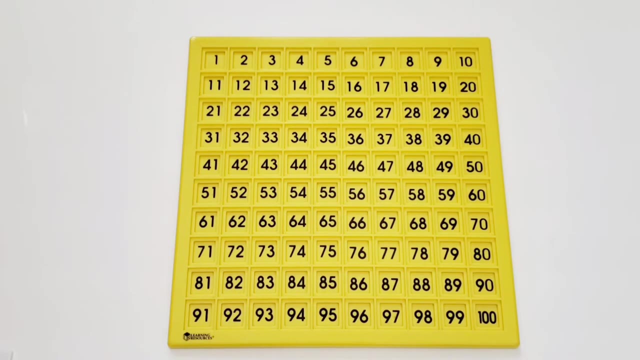 than the 66. so that means the 81 is bigger than 66. so this time we're going to point our arrow this way. okay, I hope that makes sense. now we're going to start working on the concepts of addition and subtraction, and so, to start that off, we're going to just talk about the concept of adding on. 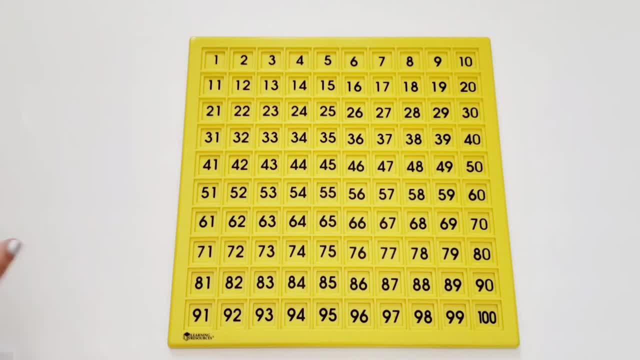 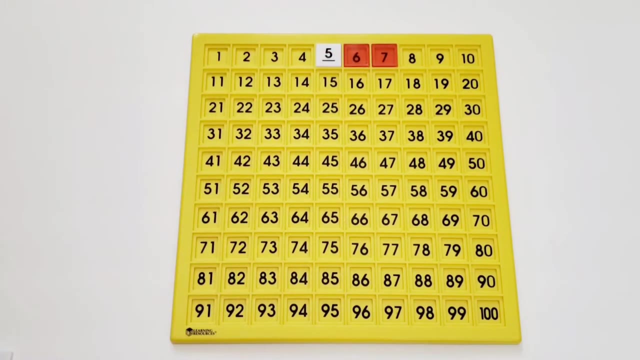 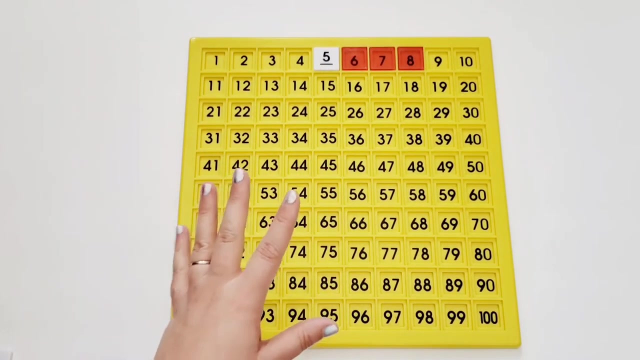 or taking away. so let's start with some easier numbers. here's the number five, so let's talk about adding on three. so let's add three tiles here and we will find that our answer is eight. five plus three more equals eight. it could also be the other way of: how many do you need to get to eight? okay, 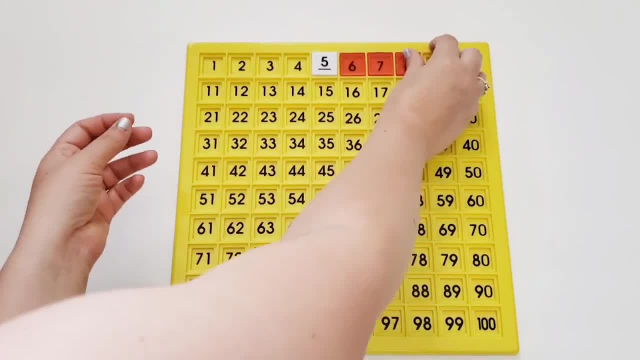 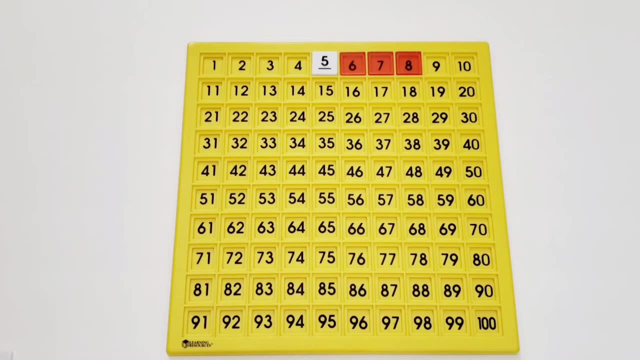 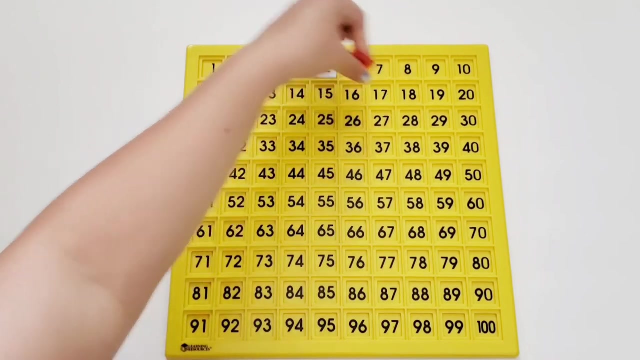 and so we'll know that we just need to keep placing until we get to the number eight, and then we see that there are three red tiles there. so five plus three equals eight, and then the same way for subtraction. so let's take away three, this time five. take away three loops, let's take 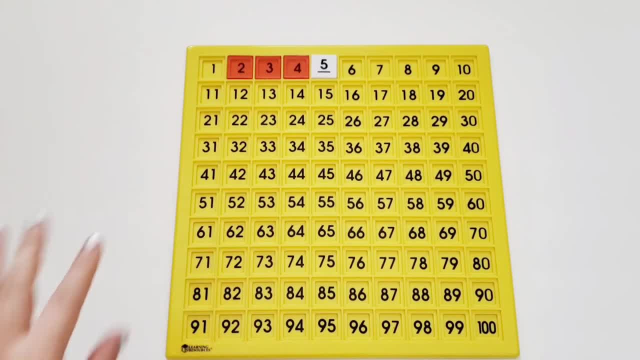 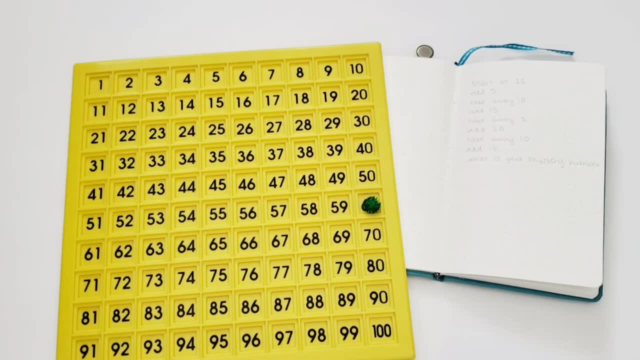 away three and our answer is two. okay, real simple. adding on and taking away- real simple. this next activity is one that Michael did at the end of his last school year, and we had to pull out our hundreds board to make it a little bit more interesting. so what he had was a worksheet, which I don't currently have anymore, so I just kind of made 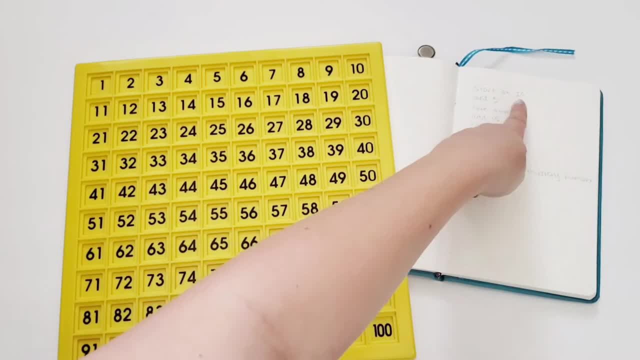 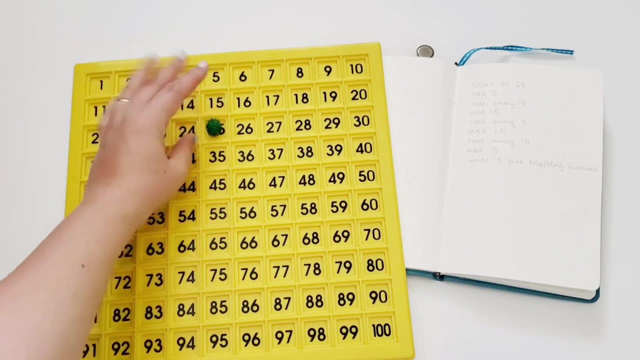 one up for you over here. that was the same concept. so what you do is start at a particular number, and so I'm just going to use a little pom-pom with a magnet on it. the magnet does not work on here, so that doesn't matter, but just use whatever counter you have to put in your designated starting point. 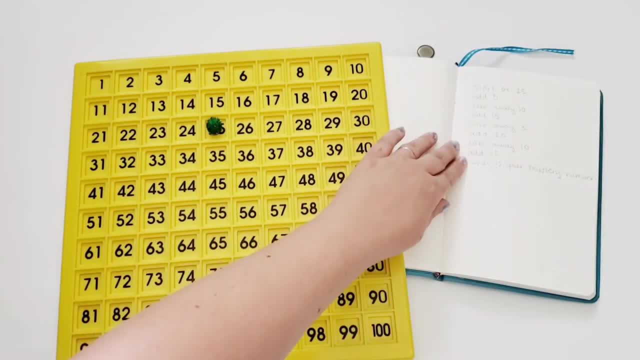 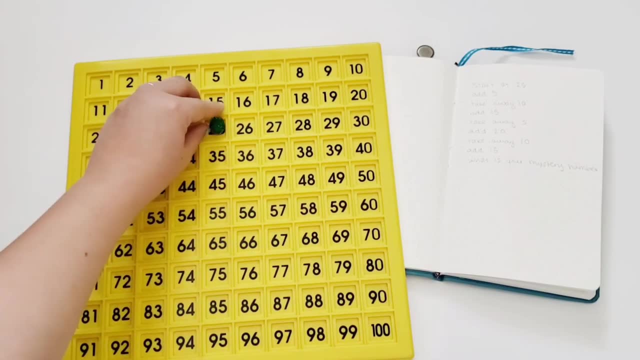 so our number is 25.. and so now you're going to go through the number maze or just follow the list, um, follow the instructions until you get to the mystery number. so now we're going to add five, then we're going to take away 10. then add 15.. 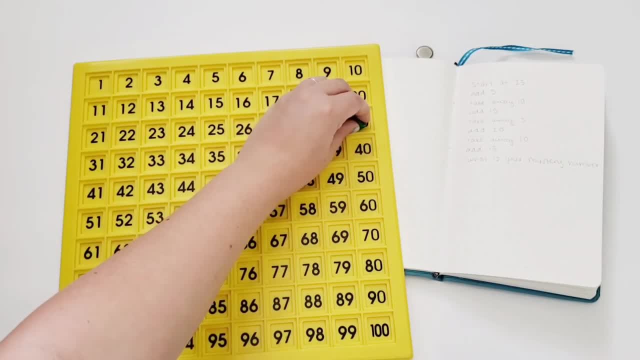 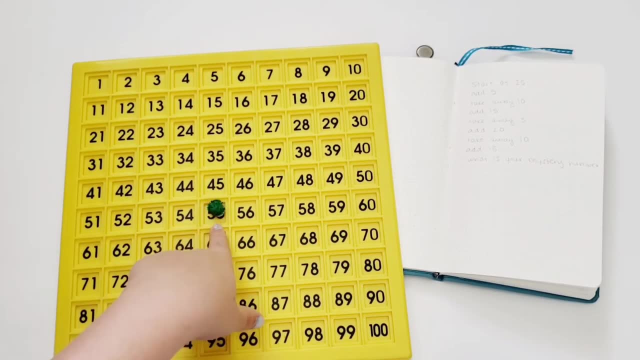 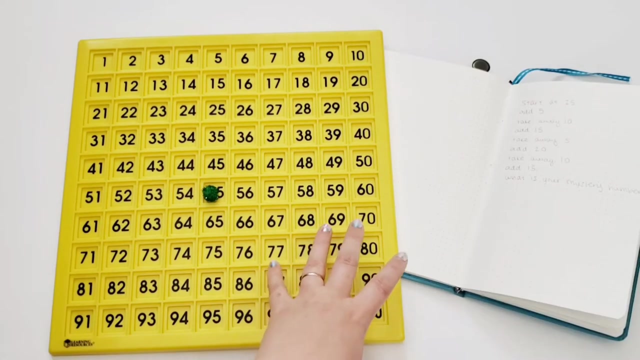 take away five, add 20.. take away 10.. and then add 15.. so now our mystery number is 55.. I hope I did all that right, but anyway, that is basically how this particular activity works. uh, doing a mystery maze, I think I've heard it called both ways- and you don't even have to follow this same type of 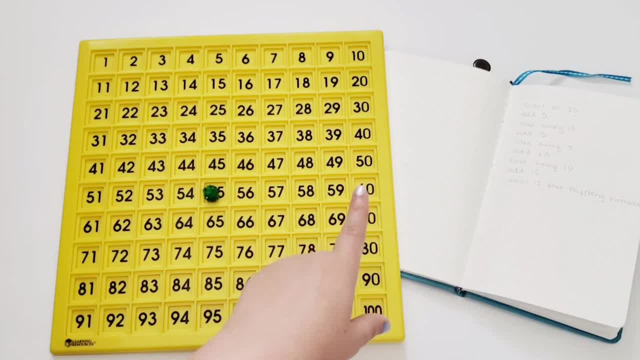 thing where they're basically going by fives. although that is a great way to connect, skip counting by fives. but you could do it with any particular set of numbers. so take away two, add 17.. I don't know, you can do whatever numbers it is you want to work with. I just remember that this. 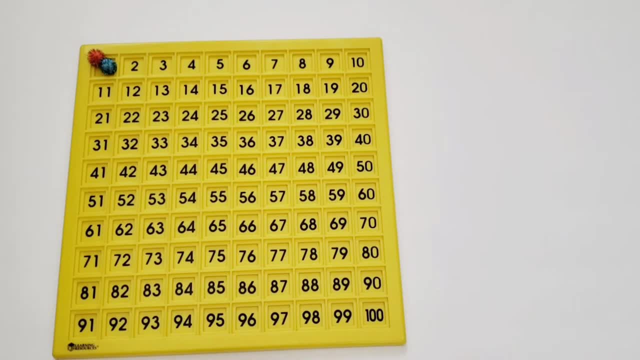 is how his was set up. this next activity you might have seen before, but this is called race to 100.. now you can do this in a couple different ways. you can play, uh, just one player by themselves, but it's definitely more fun with two players making. 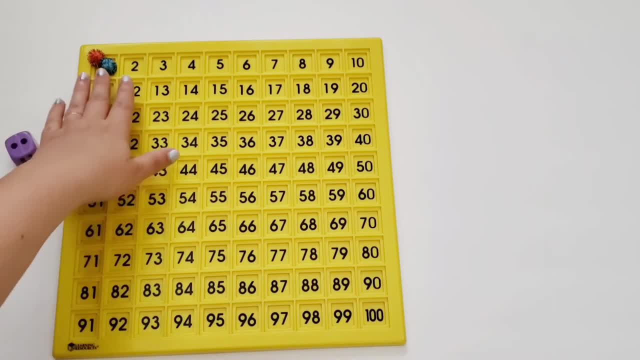 it a race you could also have. basically, what you need is a counter to move along the board and then dice to figure out how many numbers to move, and so you can either do that with one dice for each player or, depending on if it's one or two players, do both dice together to make. 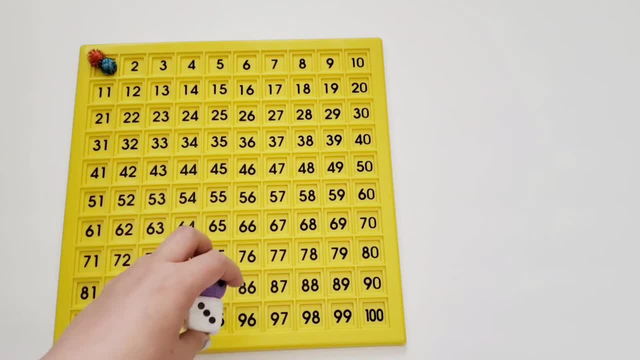 it a two-digit number that they need to move along the board, with um definitely raising the difficulty level. so it's all up to you on whichever way you choose to play um, but we're gonna do one dice for each player for this demonstration, I mean. so basically, they 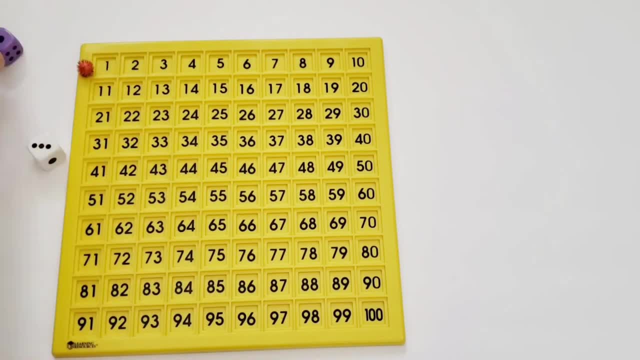 would take turns rolling how many they're going to move. so let's say, blue is, purple is going to move just one space, and then orange is going to move three, okay, and then they will just continue to do this along the road. um, I'm already forgetting what I'm doing here, but you'll see, you understand. 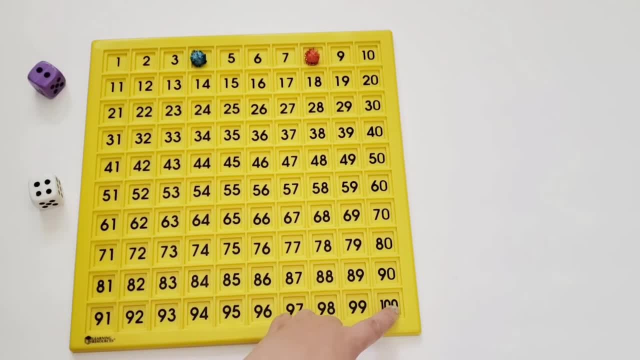 they would eventually work their way all the way down to 100, and whoever gets there first wins the race again. if you wanted to do this, um, with double, double digit numbers, um, now orange has to move five space, one, two, three, four, five. I don't know why I had to actually count that out. um, and then now. 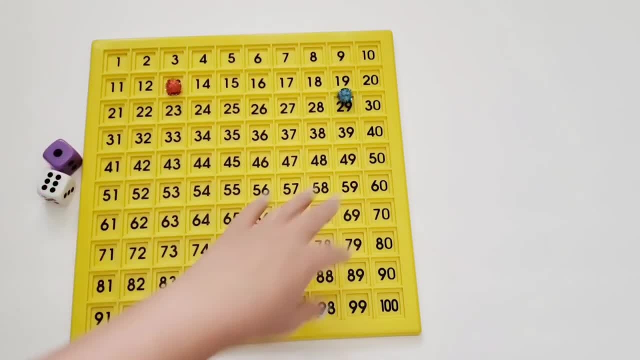 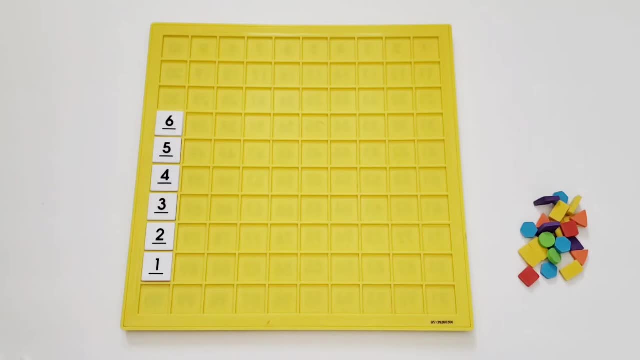 blue has to move seven. okay, whatever, okay, but that's how you get to uh 100 with this activity, and so that's going to be a lot of fun turning this into a game. um, fun activity you could do with the blank side of the board is create a graph. 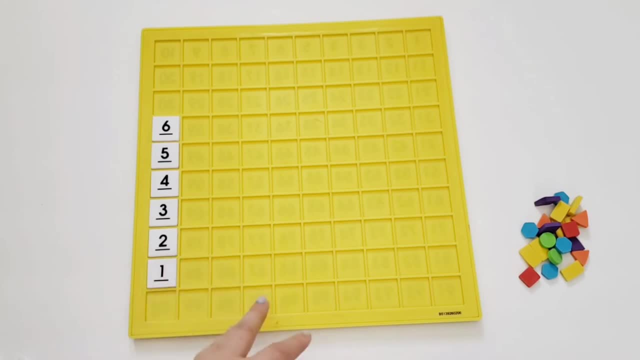 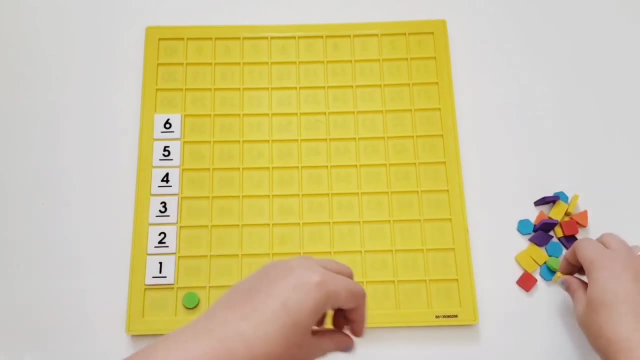 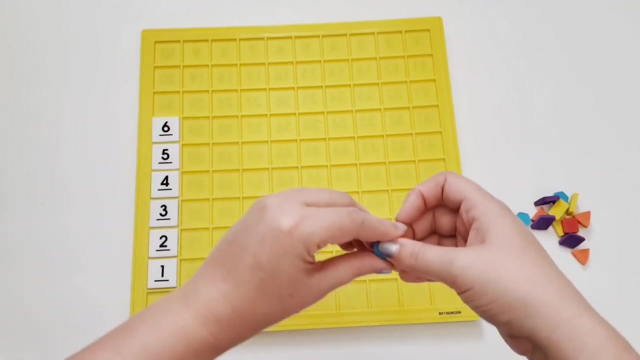 um, this might be a fun hands-on way to build a graph. so first I have one through six- that's just a random number- and then we're going to do one shape, one of each of the shapes down here along the bottom. let's see, is that all of them? and orange? okay, so now, whatever they have left, they're going. 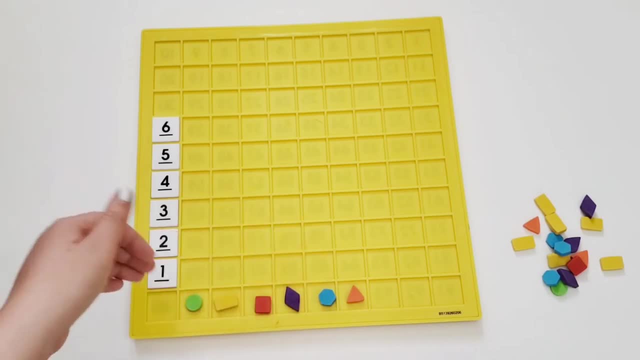 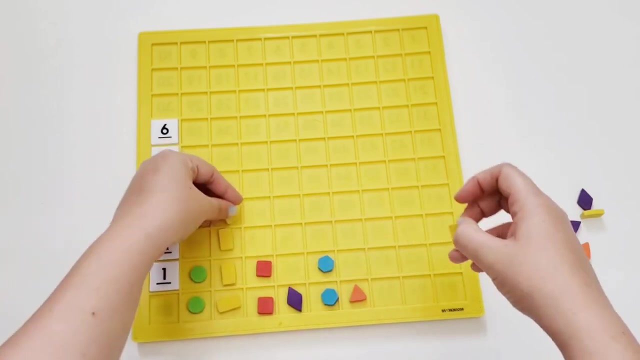 to plug this into their graph, and so now they're going to see that they have one green circle, okay, and one red square, okay. we're going to plug this in all the way and then we can discuss what our results are, now that we have our graph filled in. now let's talk about the results. 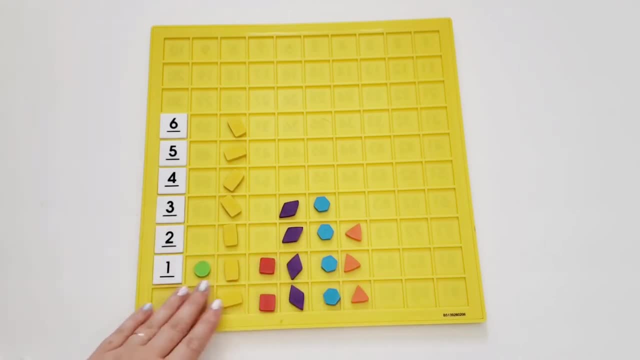 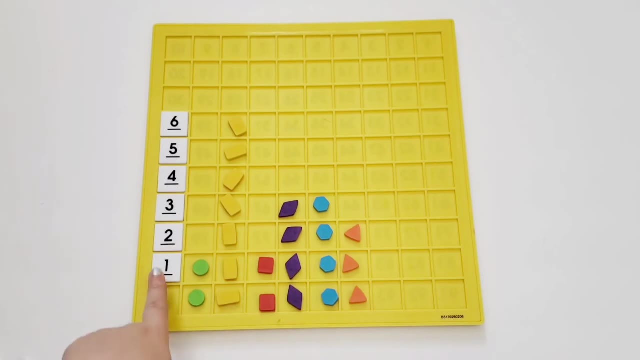 um, so we have to explain that this bottom row does not count. we're only going from the numbers across. okay, so pretend there's a line here, but we need to make sure that they understand that we're going from the numbers up. so first let's talk about how many green circles are there. there's one. 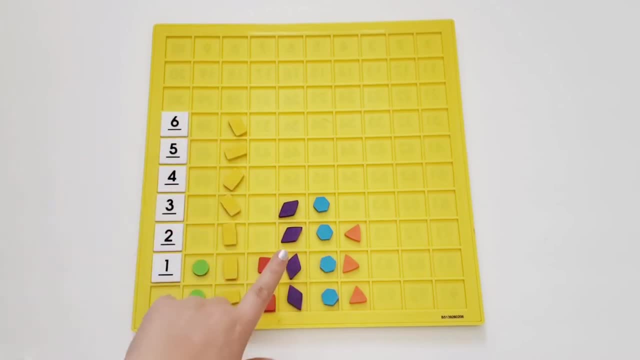 and how many yellow rectangles? well, there's six, okay, and we're going to talk about that. then let's connect a past concept that we talked about. let's talk about greater than or less than. which number has the greatest amount of shapes? well, we can see that the number with the highest 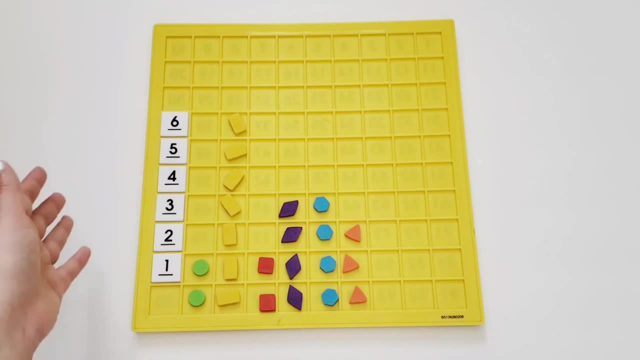 or the shape with the highest amount is the yellow rectangles has the least. Well, it's actually a tie, because we have one circle and we have one red square. That's a tie. What's another word for tie if we're talking about greater than or less than Well? 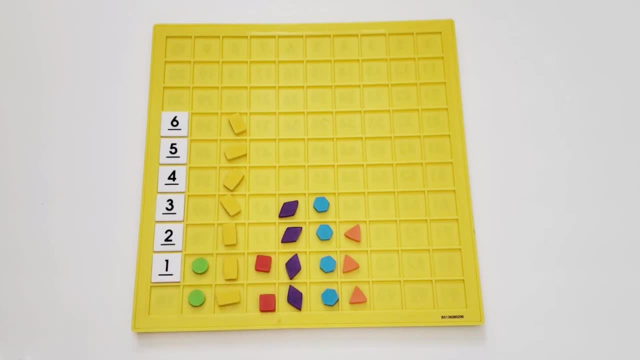 that's, you know, equal to or the same, as They have the same amount, okay. And then even these two, they have the same amount. the purple and the blue, They both have three, And then we have the two with the orange. Okay. so let's talk about greater than or less than. Let's read our results. 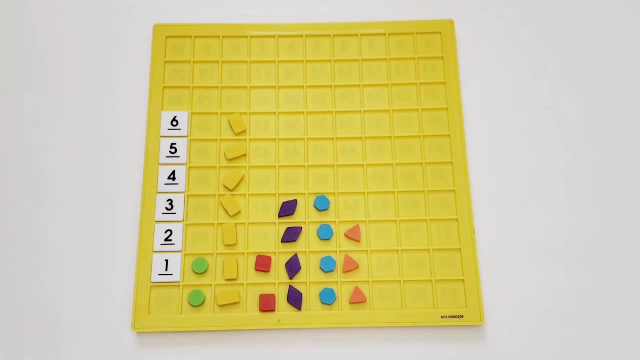 and all that sweet stuff You can even do. well, how many more of the yellow rectangles are there than the orange triangles? How many more are there? And then they can then count how many spaces So yellow has, one, two, three, four more than the orange triangles. So I just think this: 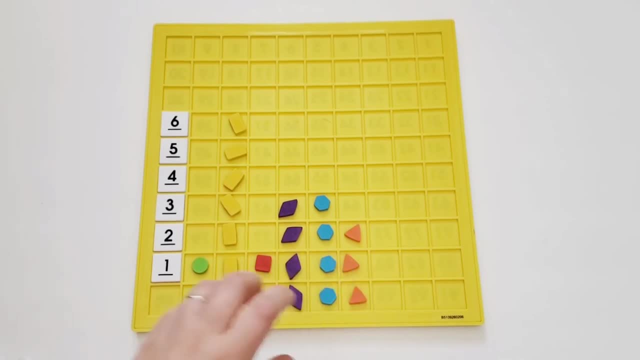 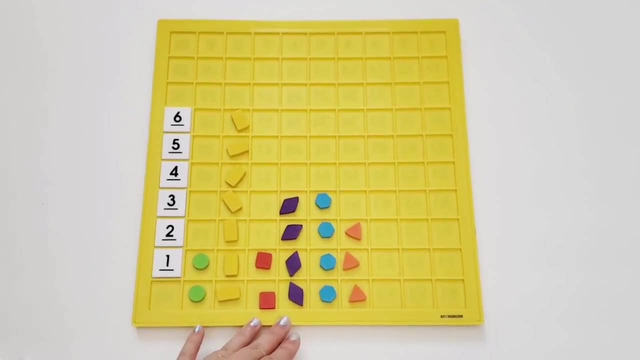 is another fun way of making this hands-on, this math concept that could be tricky, and turning this into more fun than just filling out a workbook. So it's another great use of the blank side of the board, One concept that Michael has been working. 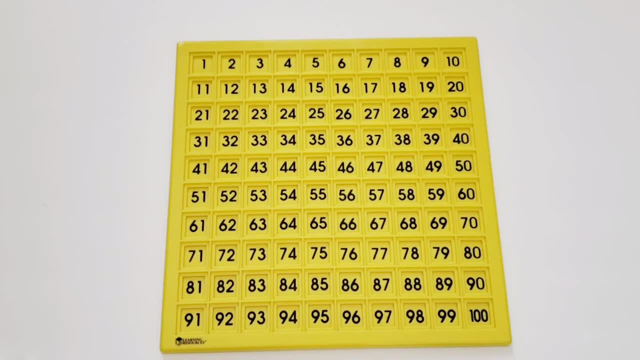 on lately in school is rounding- okay, Rounding numbers, And so I am the type of parent that likes to provide hands-on learning experiences for him when he needs extra practice. So in school he just was not fully understanding this concept, And so this is a great time to pull this out. 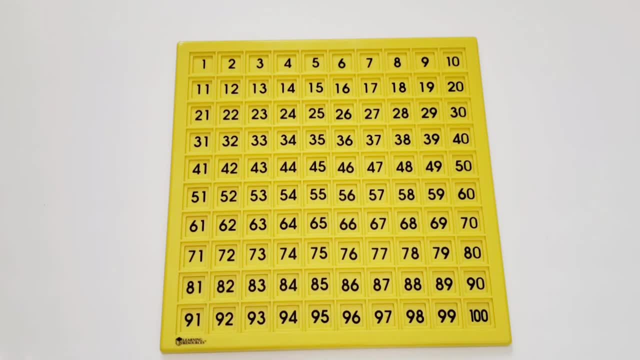 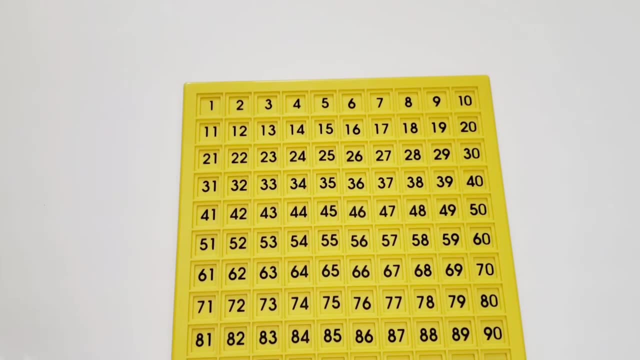 and really help him understand what he's doing. So I'm going to show you how to do that, What we're talking about. So first let's start real. simply at the top of the board with single digits, We're going to round numbers, So what I like to do is show half of the line Again. 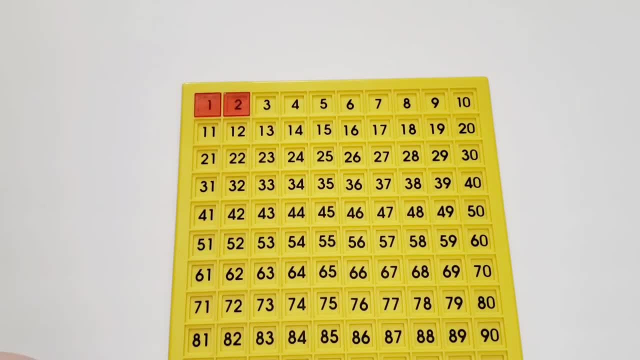 we're only doing the top line here. Let's do half of it in red, So one through five, and then the other half in blue. Now, when I did this with him, I also wrote out number lines for him, And what I did on the number line was one through five. I colored. 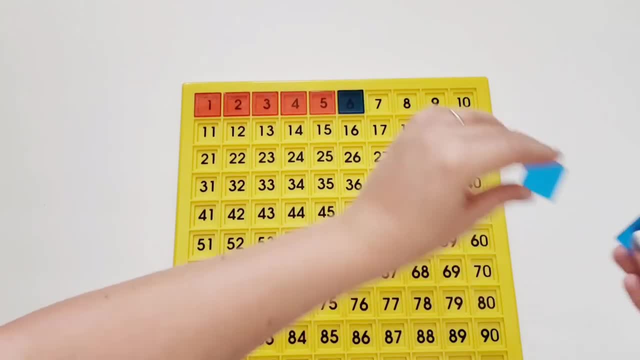 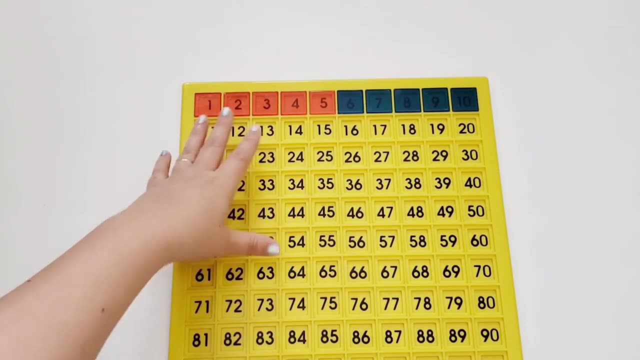 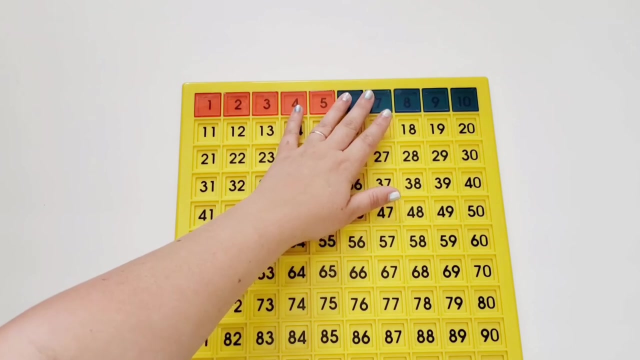 red and then six through 10, I colored yellow. So this is the same concept as if you were to write it out on a number line, but we're using our hundreds board here. So half of the line is red, half of the line is blue. So that's going to show whether you need to round up or round down. 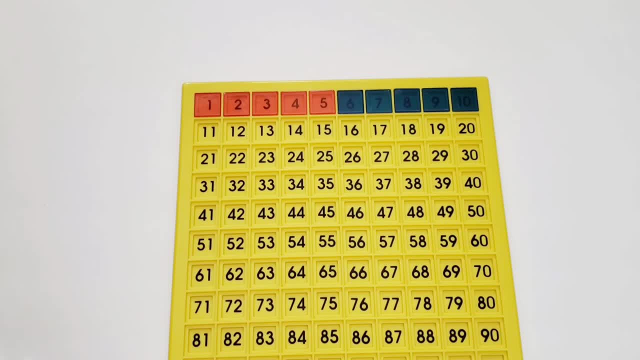 So now our number is- let's say our number is seven. We need to know: does seven round up to 10? Or does it round down to one or zero? And so we know that, since it's in the blue, that means we have to round up to 10.. Okay, so when they plug in their answer, they know. 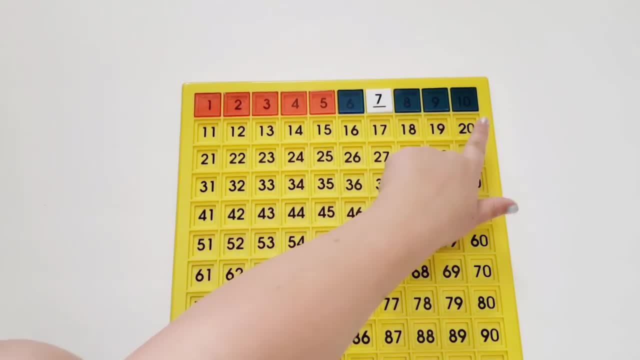 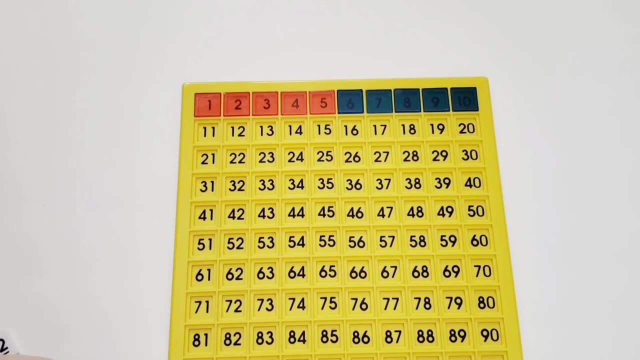 that seven, because it's in the blue area, automatically has to be rounded up. Okay, if we were to do the number three, I don't have that tile right now, but if we were to do the number three, then we know that because it's in the red, it automatically. because it's in the 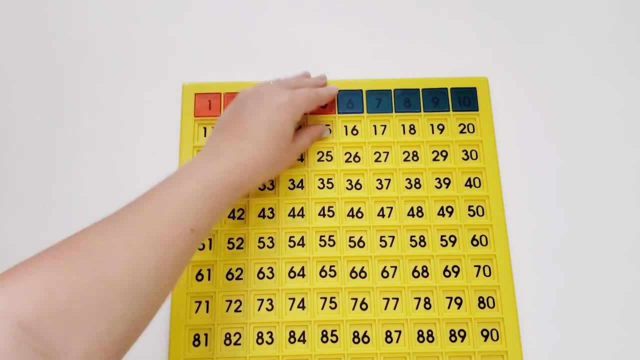 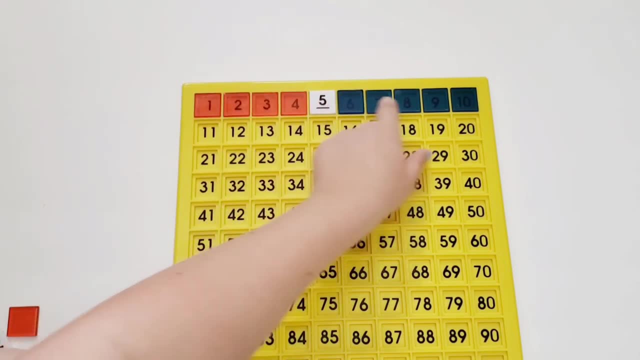 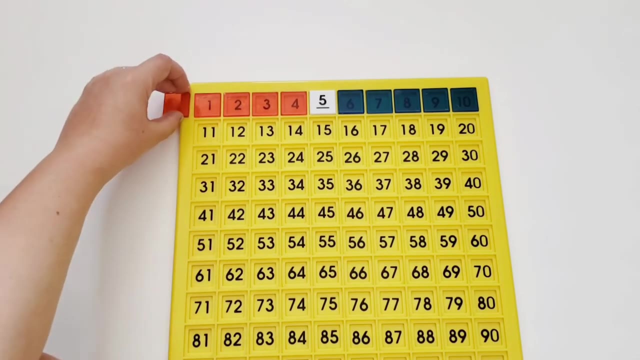 blue, it automatically has to go down. Okay, and then if we had the number five, just explain to them that anything at the halfway point, which is the number five, automatically goes up, And so that's just a concept that you'll have to teach them. One thing I do wish is that I do wish it. 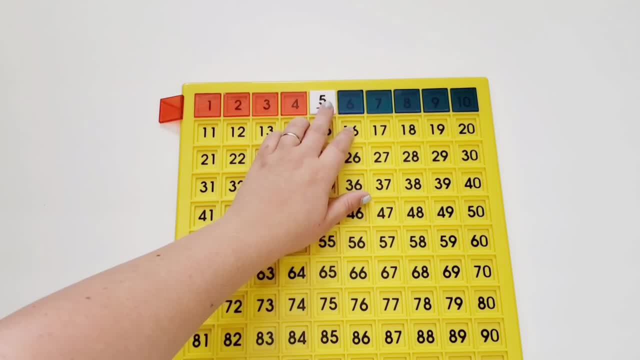 had a zero place here, because then that would really help with the five, make more sense that it has to go up. But regardless, just make sure they understand that the halfway point is always going to go up. Okay, so that was only for one through 10.. But the same concept can be done. 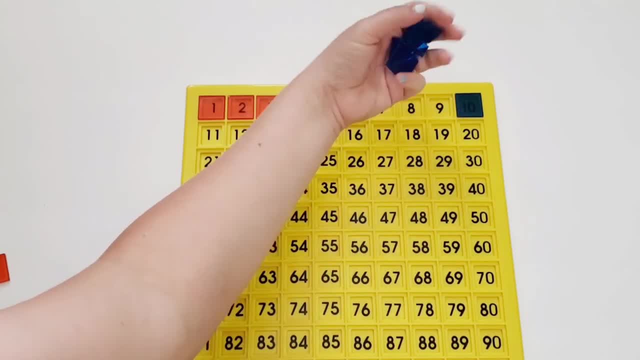 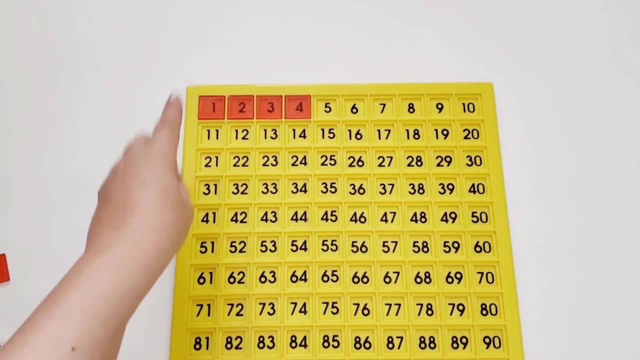 with one to 100. Or you could even do just one through 20.. So let's do one through 10 is red and then 11 through 20 is blue. Okay, but the next concept we're going to do is one to 100. So 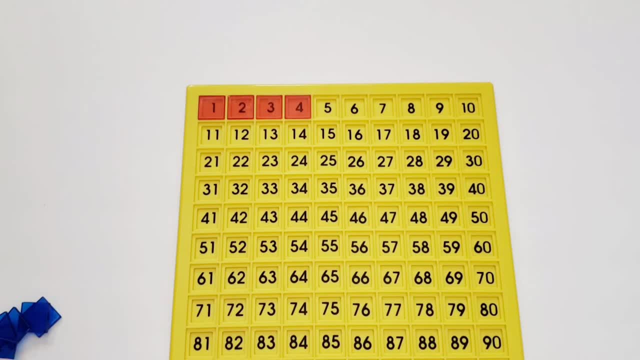 half the board needs to be red. the other half needs to be blue. Let's see if I have enough tiles for that. Okay, it looks like there's only 25 of each color, So that's fine, We'll just do one. 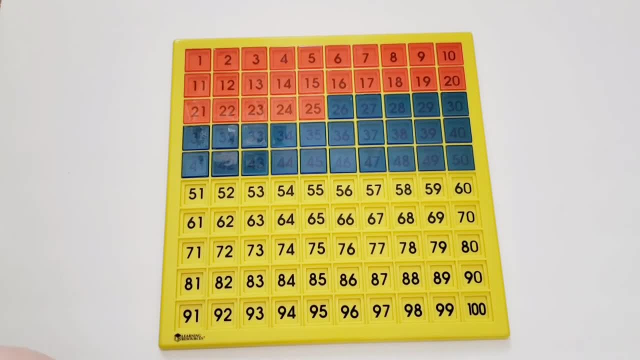 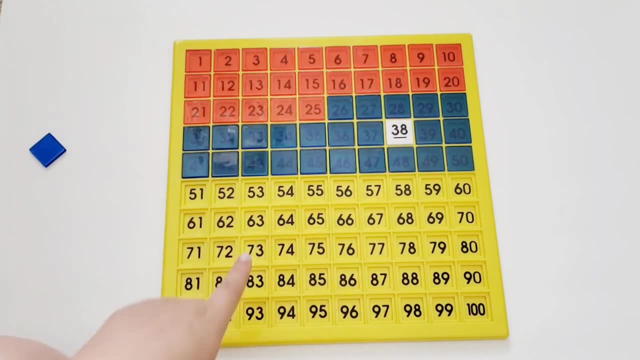 Okay, so now we're going to round whichever number we have, from one to 50. So here's 38, I happen to have next to me, So let's plug in 38. If it's in the blue section, then it automatically rounds up. 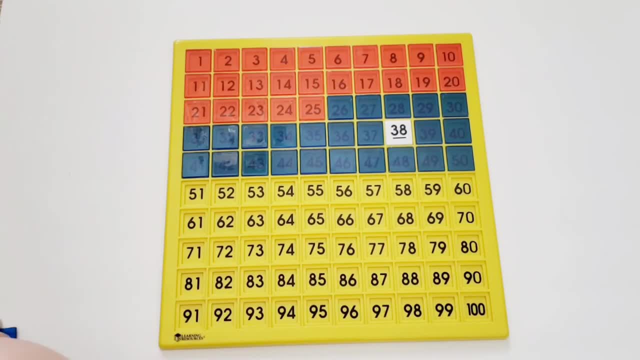 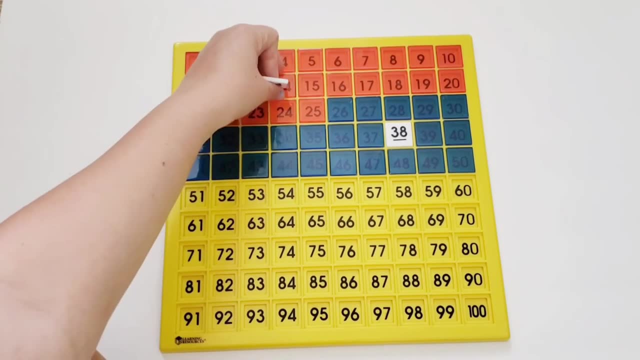 to 50.. Okay, so 38 is rounded to 50.. Same thing if we were to plug in- I don't know, let's find a different number- 14.. Would 14 be rounded to zero or 50?? Well, we know, it's a. 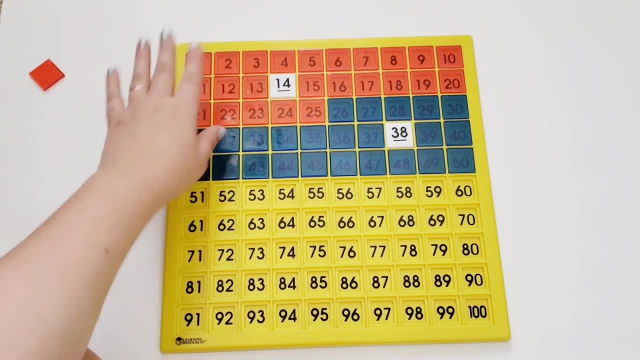 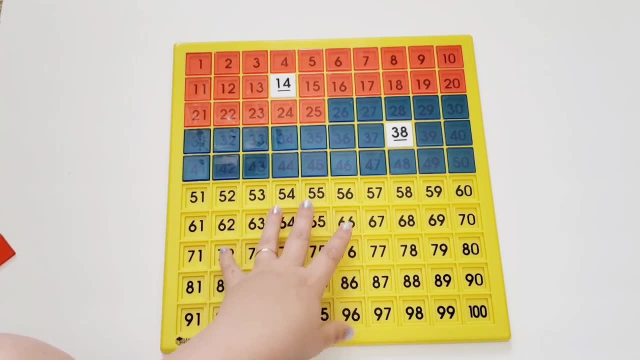 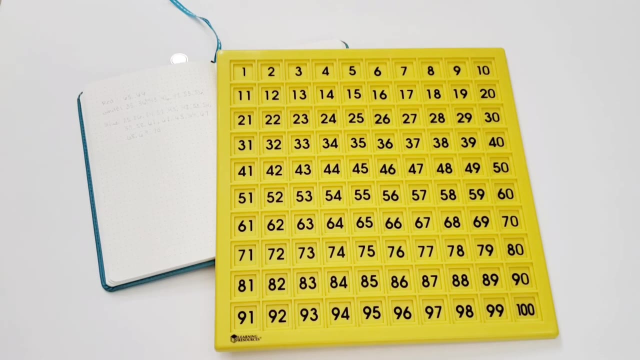 red section so it automatically goes down to zero or one or whatever numbers you're working with here. Okay, so that is how we're going to show rounding with our 100s board And to finally finish this video that has been super long is my favorite activity to do with the 100s board And 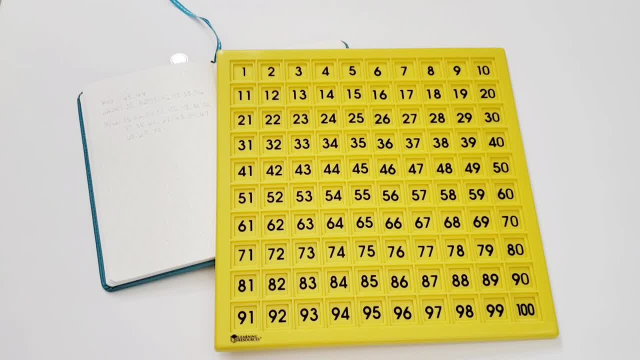 that is the mystery picture. You've seen these worksheets before. They're always fun to color them in with your crayons or whatever else, But now we're going to take it to a different level by doing it in a different way. So let's go ahead and do that. So let's go ahead and do it in a different. 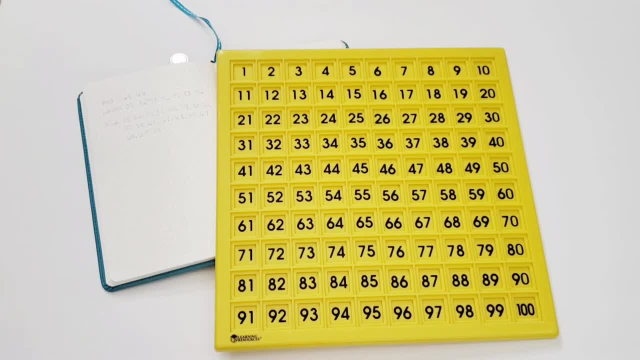 way. So let's go ahead and do it in a different way. So let's go ahead and do it in a different way, with hands-on tiles instead of coloring. Okay, so now we are going to have our three colors: red, white and blue. This is one that I have shown before on my channel, So, if you have, 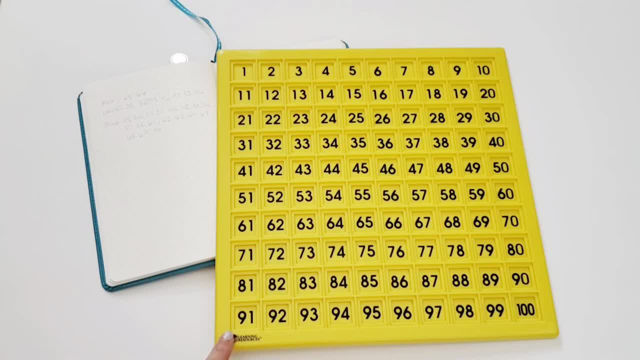 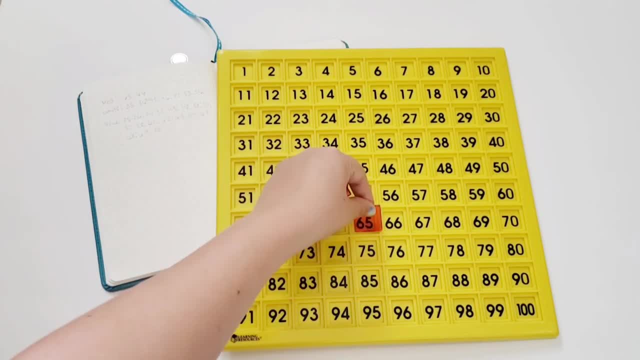 one. So now I'm just going to go ahead and show you this one. So now I'm just going to go ahead and plug in the colors. So red is 65 and 66. And we'll just go from there. So let me go plug those in and